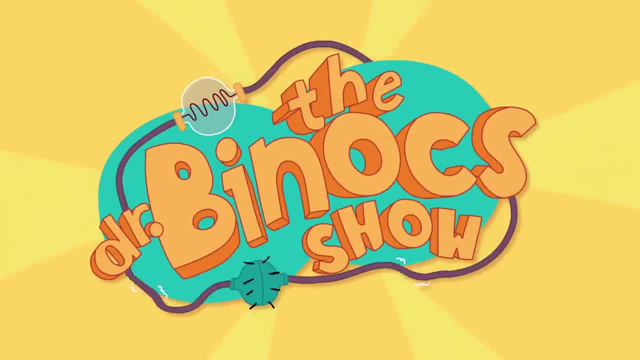 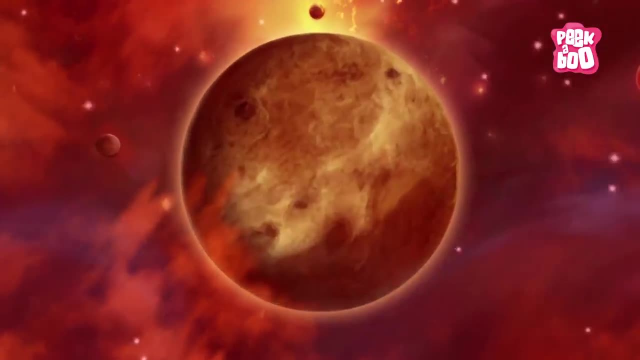 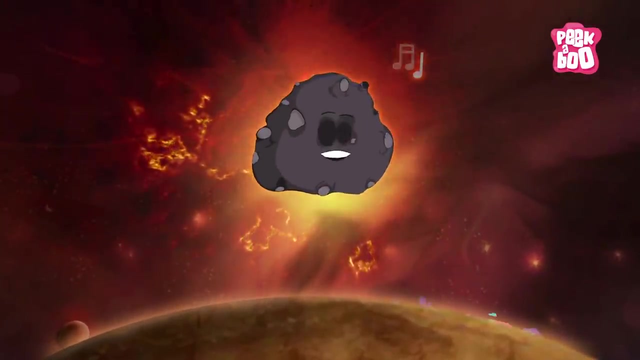 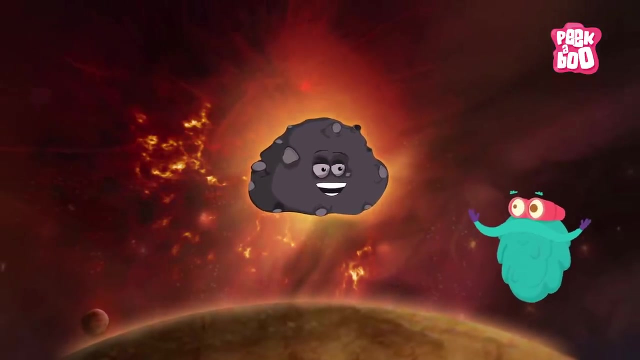 I am the meteorite. don't take me for a ride, cause I then turn into a meteor. I pass through the atmosphere of the earth. now. don't get scared, cause I then turn into a meteorite. That's right. Very well, Mr Meteorite, let me simplify your poem for my friends out here. 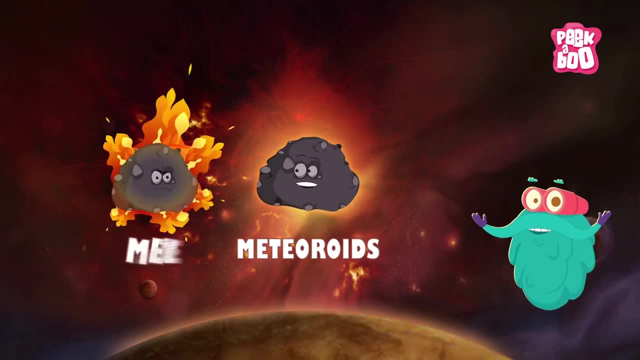 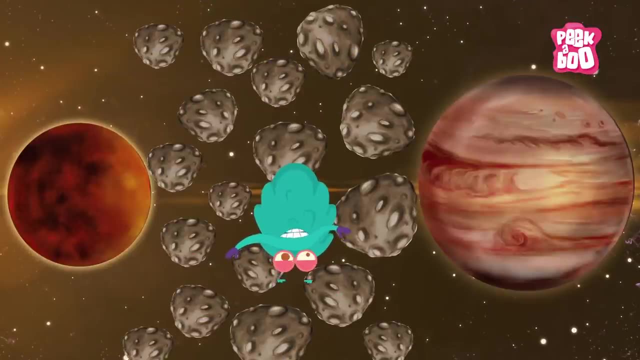 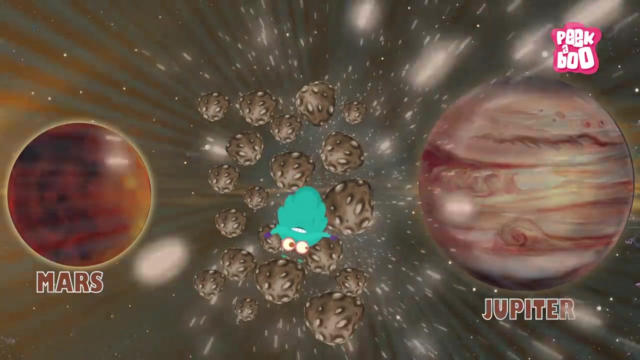 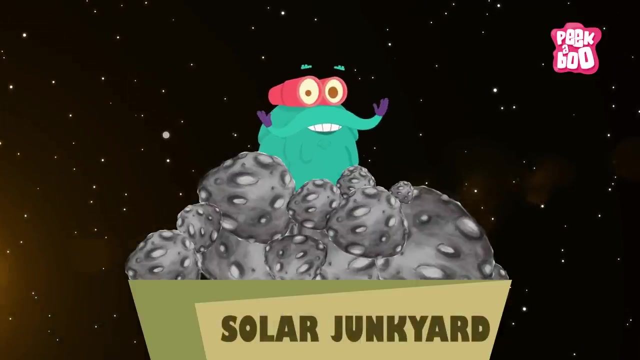 Come. we'll talk about meteoroids, meteors and meteorites today. Zoom in. A meteoroid is a small rocky solar object found in the asteroid belt between Mars and Jupiter, Yikes, Which is often known as the solar junkyard. 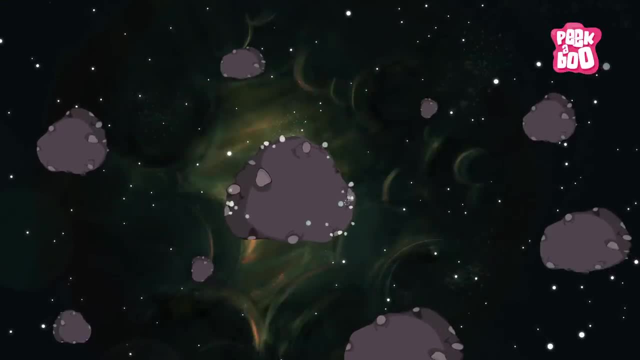 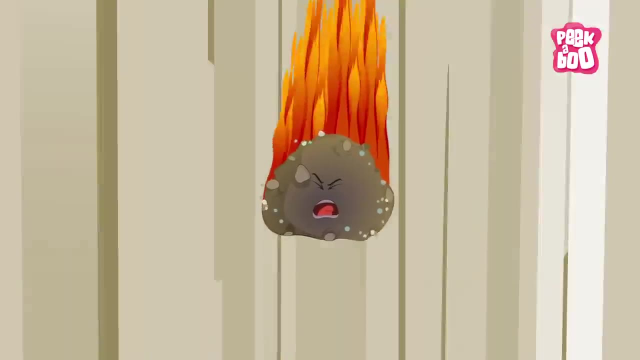 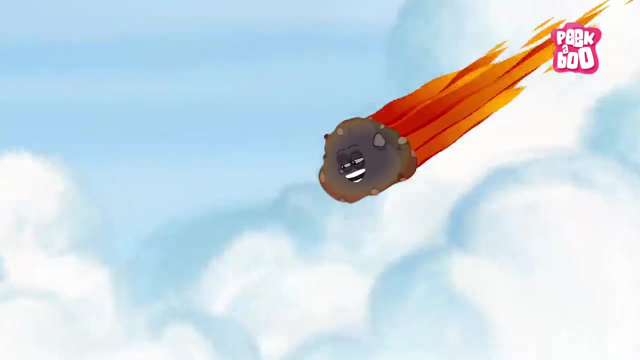 When the molecules around the meteoroids rub against each other, they start burning. When this burning meteoroid passes through the earth's atmosphere, it is called a meteor, And when that meteor survives through the atmosphere and collides with the earth's surface, it's called a meteorite. 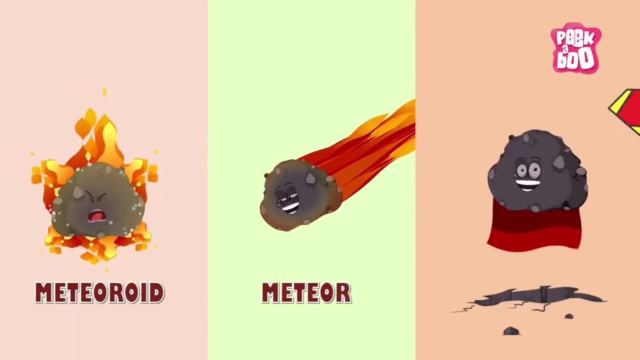 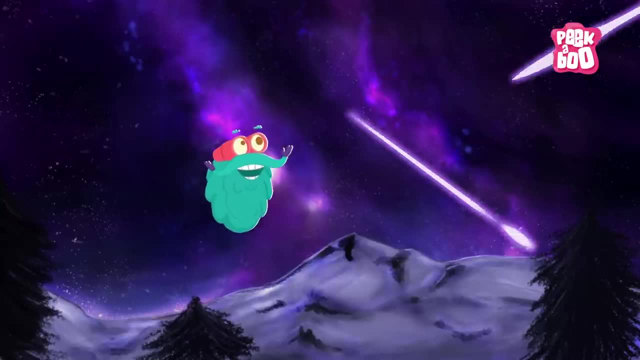 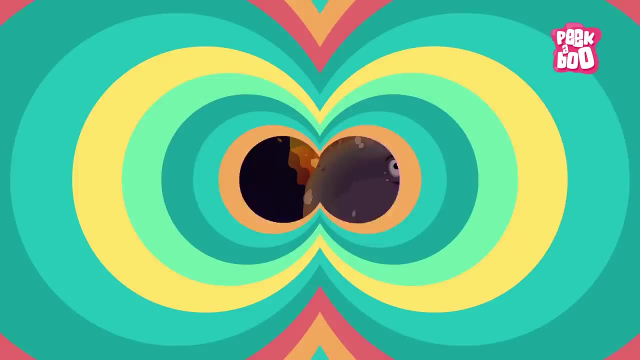 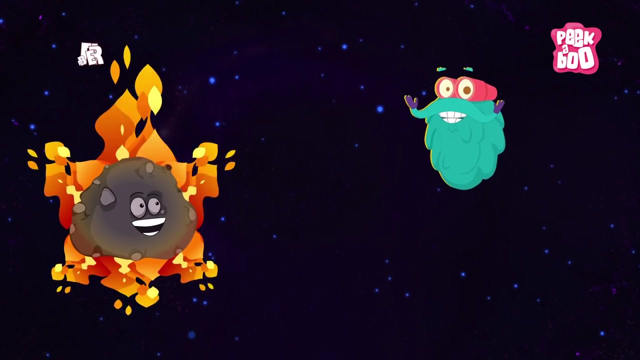 A meteoroid, A meteor And a meteorite. Haven't you seen shooting stars? Wow? Well, those are actually meteors. Some meteors burn brighter than the rest, often known as fireballs. Some fireballs appear even brighter than the planet Venus. 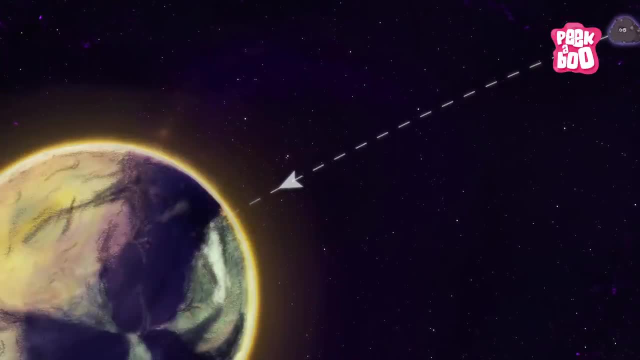 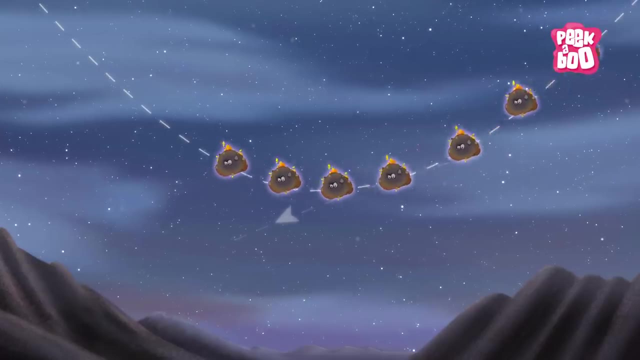 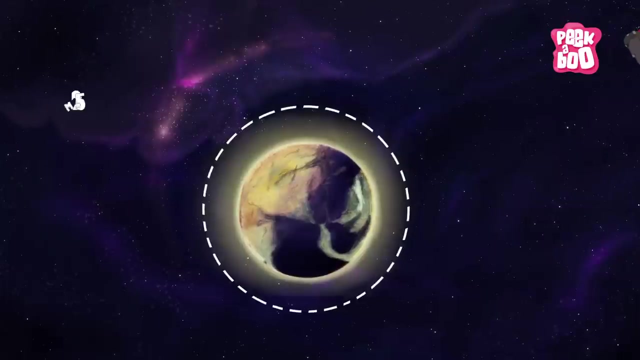 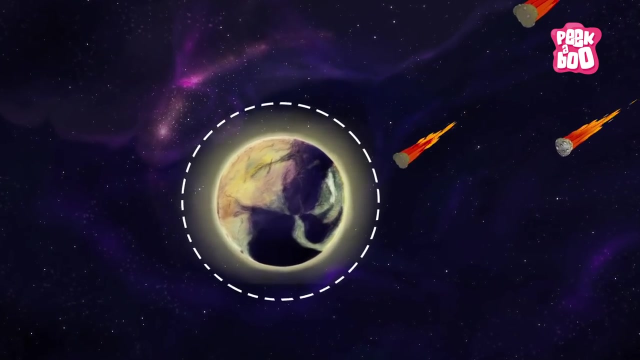 Hahaha. There's a small percentage of meteoroids that follow a particular path to the earth's atmosphere and then back out again, And they are called grazing fireballs. About 25 million meteors enter the earth's atmosphere every day, But most of them often burn up. 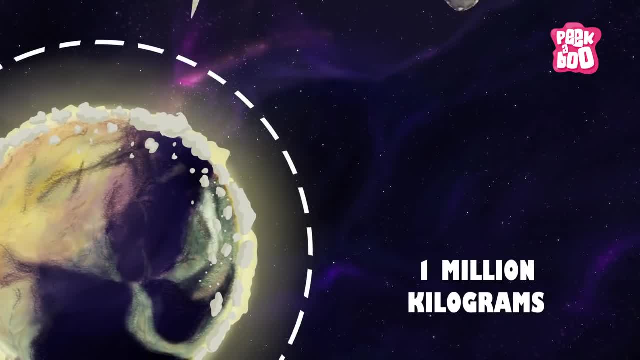 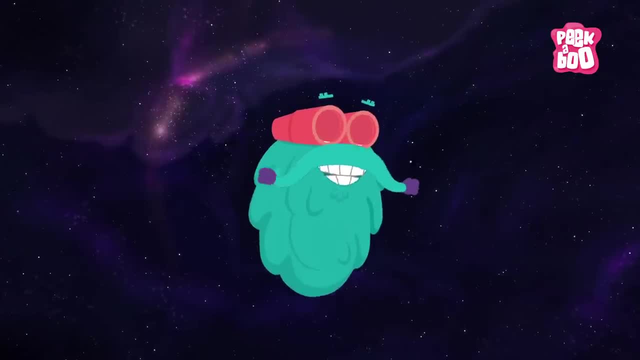 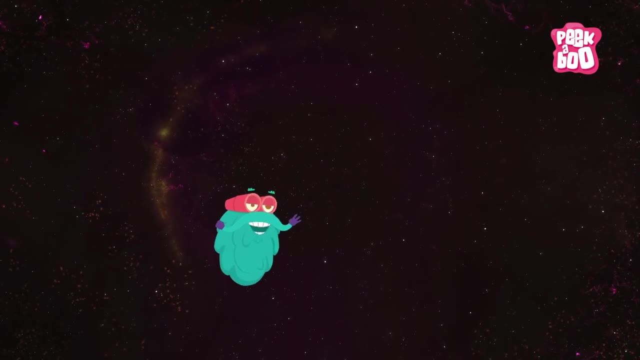 giving out 1 million kilograms of dust per day that settles on the earth's surface. So who knows, the dust around you could be from space. The meteorites are classified into three types: The stony ones, the ones that have iron in them and the magnetic ones.